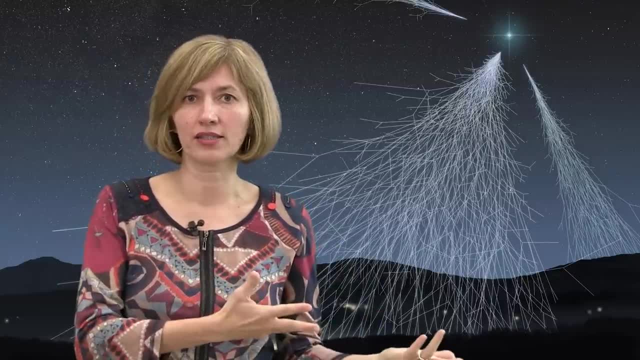 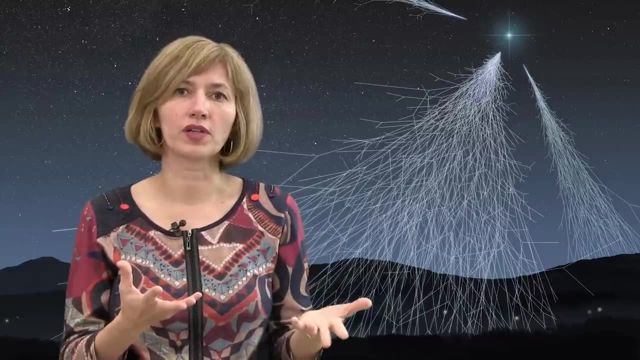 appear one way first, and then we realize that there's something else. So these cosmic rays- actually not rays, they're particles. So they're one of the most energetic particles we know in universe, and they accelerated to those energies or those velocities by some mechanism, The way 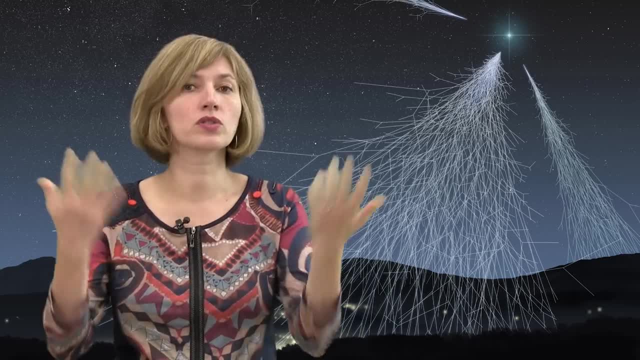 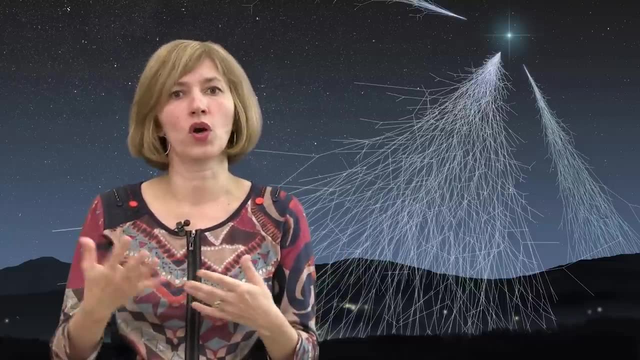 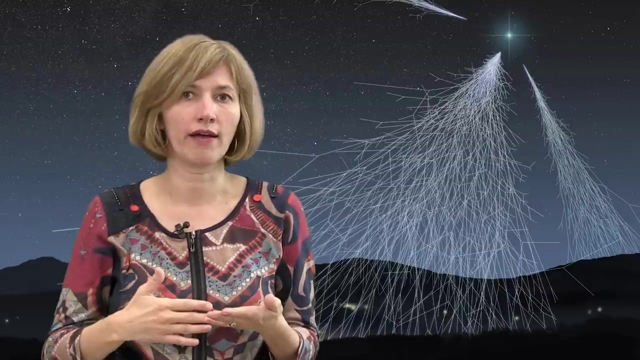 they were discovered is that they were the balloons. the scientists were sending balloons up in the atmosphere and they would have photographic plates or other means of measuring what's going on, and they noticed these particles and they noticed that the amount of particles increasing as the balloon is going higher up. So, although we discovered them 100 years ago- 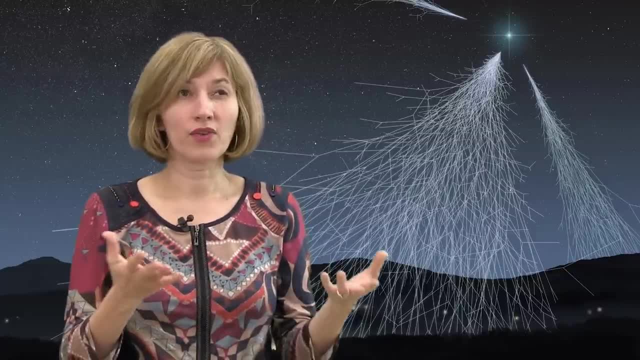 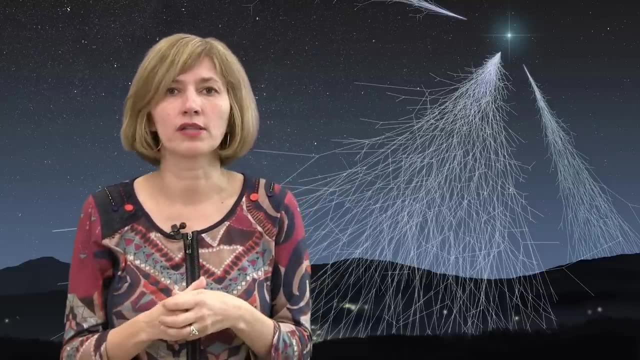 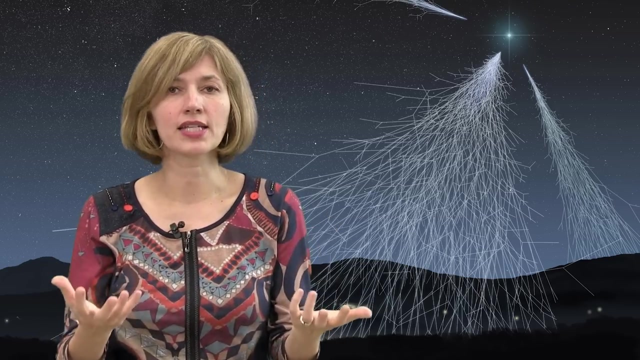 we're still not sure. We're still not sure what's producing them. The reason is because they charge particles Mostly. they are very ionized atoms, nuclei of certain elements, and they're mostly positively charged. What that means is that, as they're released, from whatever source is creating them, they have to follow magnetic field lines of interstellar medium. Between the stars within the galaxy we have what we call interstellar medium, which is very low density but it has magnetic field and as those charged particles are released they sort of get locked in and 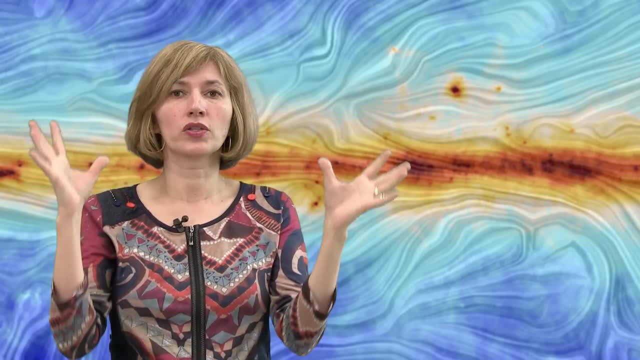 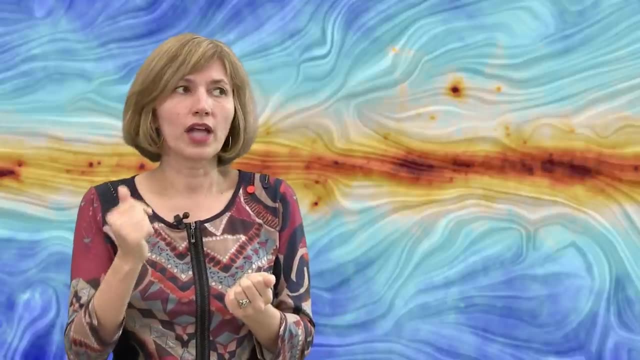 follow the path of magnetic field lines. So if we were to look at the sky and detect cosmic rays, we would see them coming uniformly from all over the sky. So then we look at the energy requirements. What could be so powerful to create these particles, And one of the most? 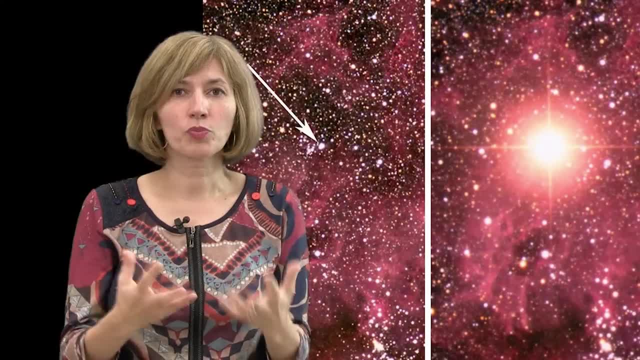 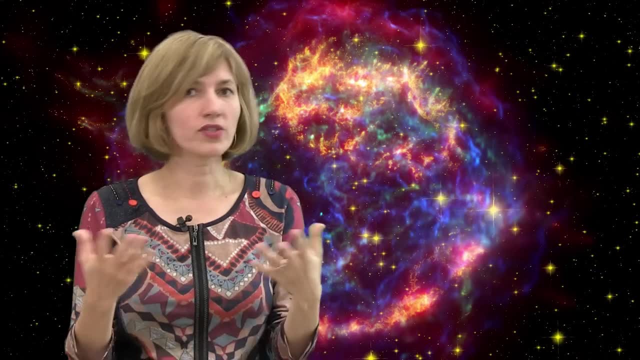 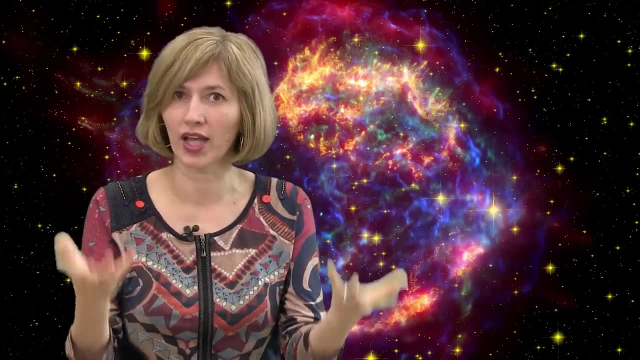 obvious sources are supernova remnants. Supernova remnants are remnants of supernovae, And supernovae are explosions of massive stars. As you probably know, the way our sun creates energy is by fusing two hydrogen nuclei- sorry, four hydrogen nuclei- into helium nuclei And in 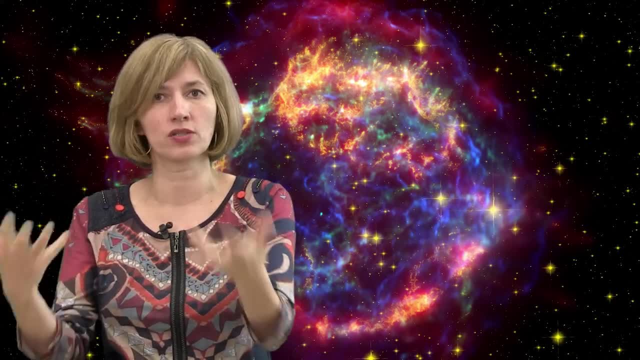 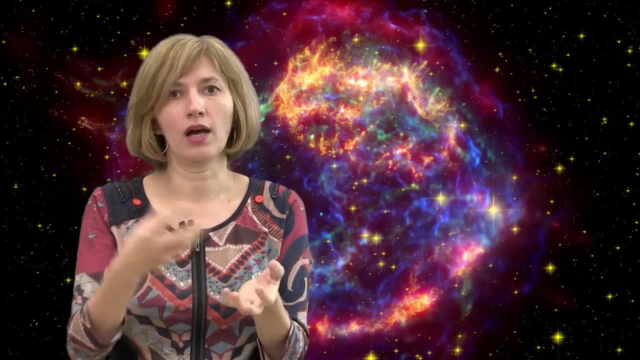 that process, some mass is lost and that mass is the energy that is released. that gives us energy from the sun, And stars, like our sun, burn or fuse, then helium to carbon and that's where they stop. They don't have enough mass to create temperature in the air, So they're. 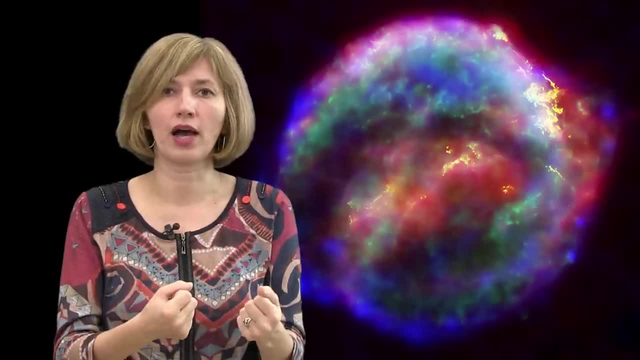 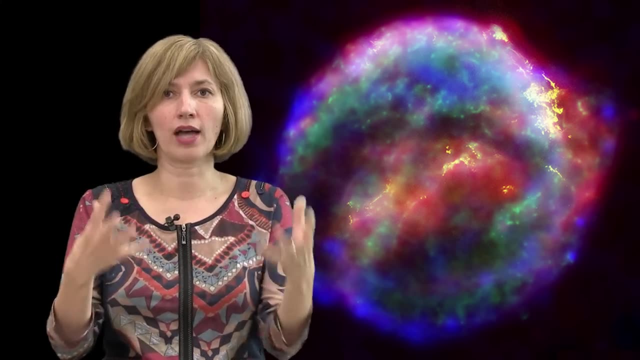 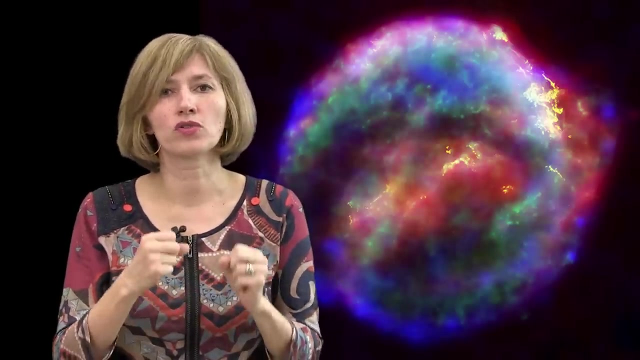 able to create temperature in their core to be able to burn carbon, But more massive stars, those that are eight or more times bigger than our sun, they can actually fuse carbon into the next element, all the way up to iron. The reason they stop at iron is that iron is one of the most stable elements in the universe. So it requires more energy to be fused together than energy released. So these reactions by which stars produce energy basically become inefficient once the core of the star is full of iron And this is where the thermonuclear reactions stop. 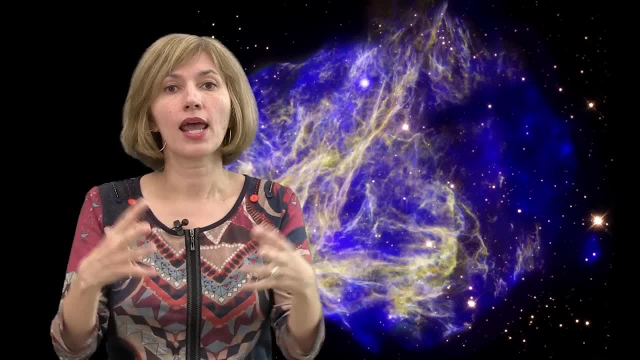 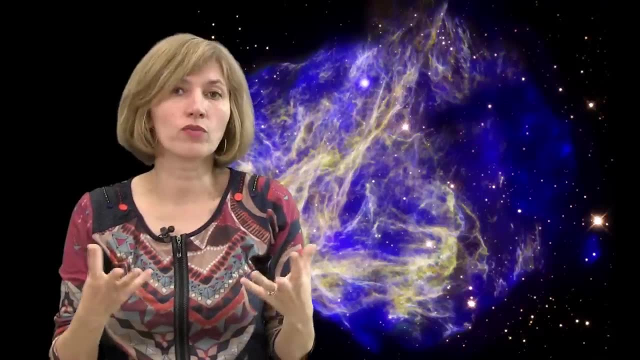 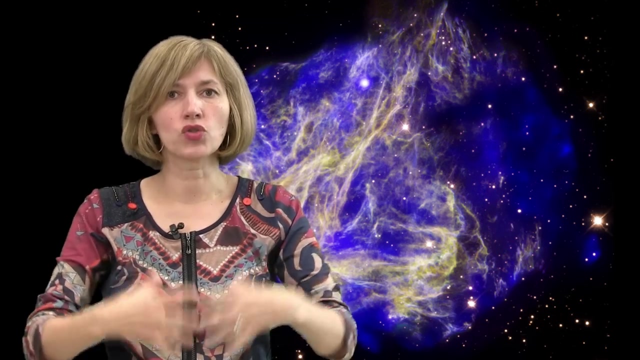 these reactions of fusing elements in higher elements And the gravity of the star pour everything down, and then the shock is created and bounces off. This is one of the most energetic events in the universe and therefore we could imagine that this is the energy needed to then. accelerate the particles So, as the shock bounces off the core of the star, the remain core of the star, which usually creates neutron star or, in some cases, black hole. this shock travels and creates beautiful shells that we call supernova remnants. They come in various shapes and sizes. 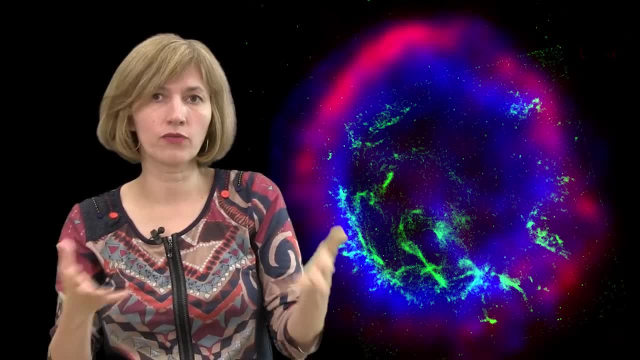 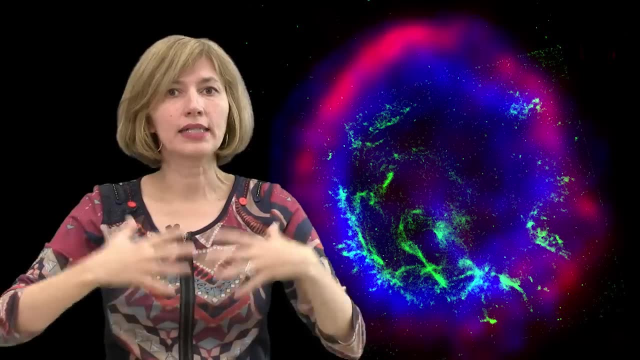 and they usually live about a million years. And by live we mean we are able to detect them, we are able to see them. So in this process, as these shocks are traveling, basically they're able to sweep the material in front of them and compress magnetic field. As they're compressing. magnetic field in the interstellar medium. the particles that they sweep in their shock shells are basically then accelerated by passing back and forward through magnetic field lines And at some point they gain enough energy to leave the source, to leave this shell of supernova remnants. 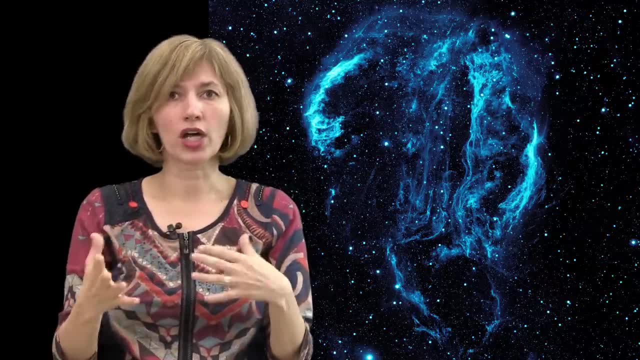 That's the theory. In practice, we are struggling still to prove this connection, mostly because the data that we need to prove this are still not, of course, available to us. So we are struggling still to prove this connection, mostly because the data that we need to prove this are still not of. 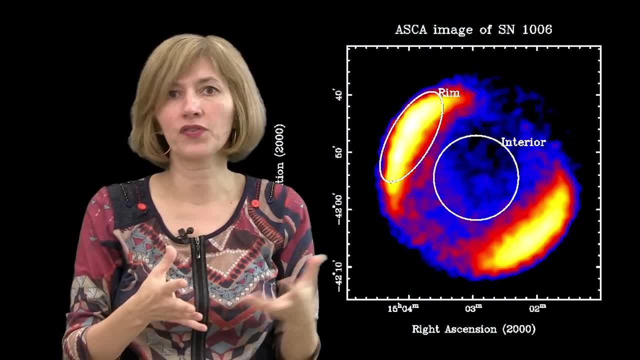 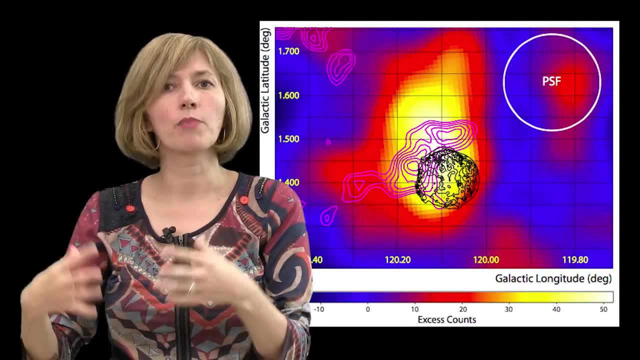 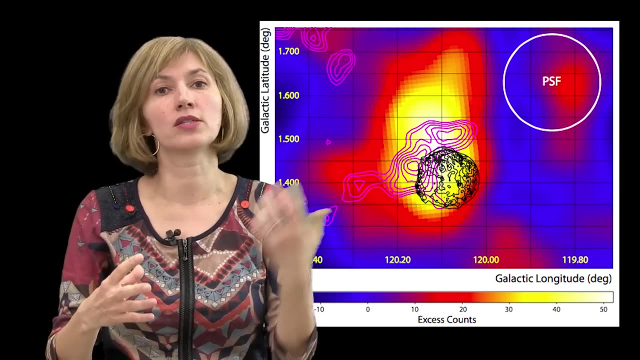 high quality We just detected. about 15 years ago we just detected some of these particles in x-ray energies And now we able to detect them in gamma rays as well. but gamma rays still have quite low spatial resolution. So when we compare pictures of supernova remnants in 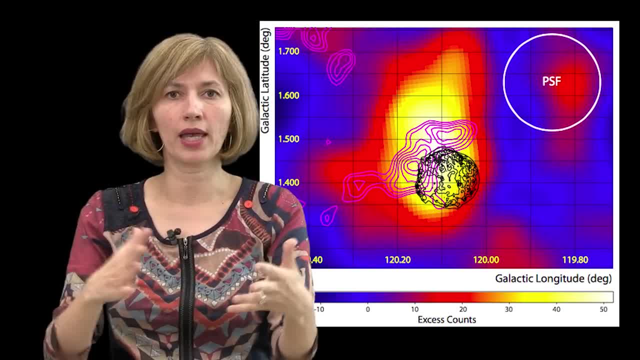 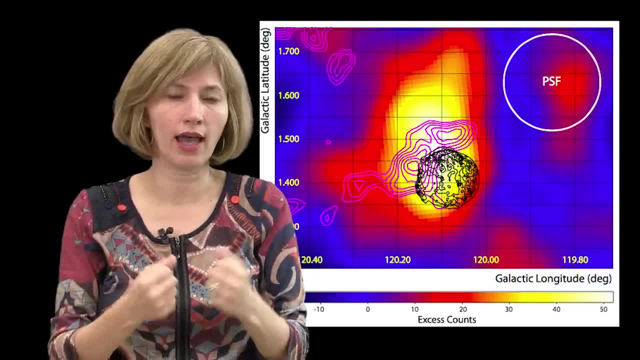 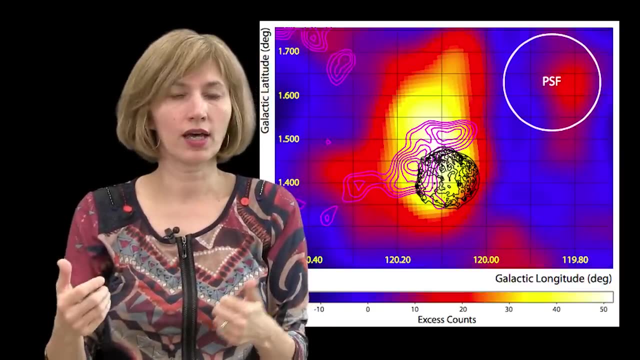 optical and radio and x-ray with those of gamma rays. we can't make too many comparisons. So this is where the science of cosmic rays is at the moment, And we basically rely on getting better and better observations and better and better telescope to actually prove this. 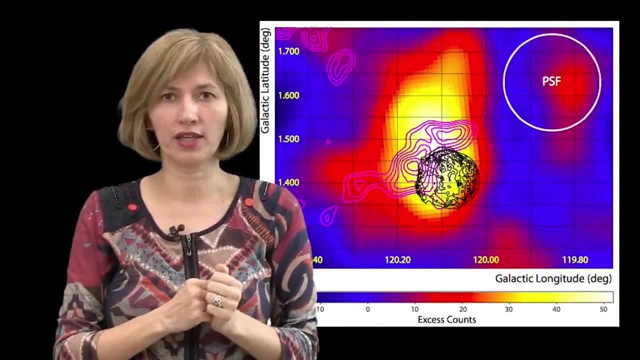 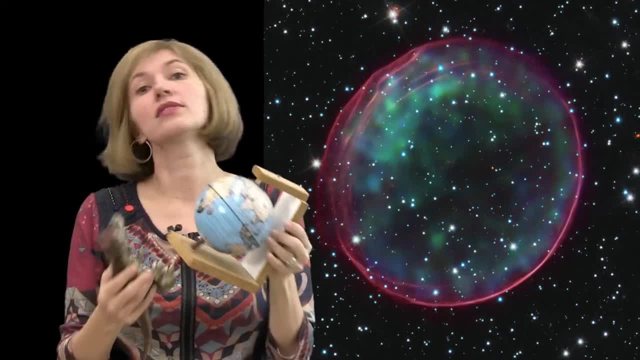 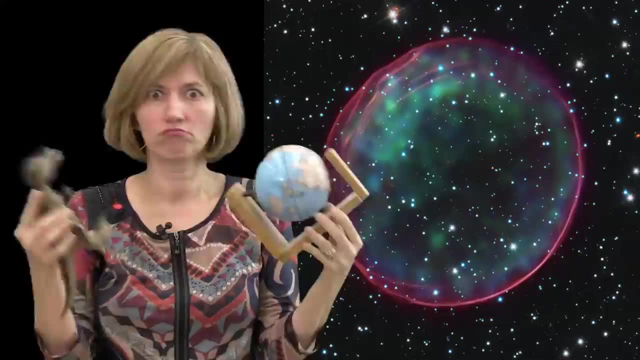 But cosmic rays, being mysterious, are often blamed for different things. One of the things they were blamed was that they killed dinosaurs, But that's discredited. Another thing was that they are responsible for global warming, But that's discredited as well. several times not working. 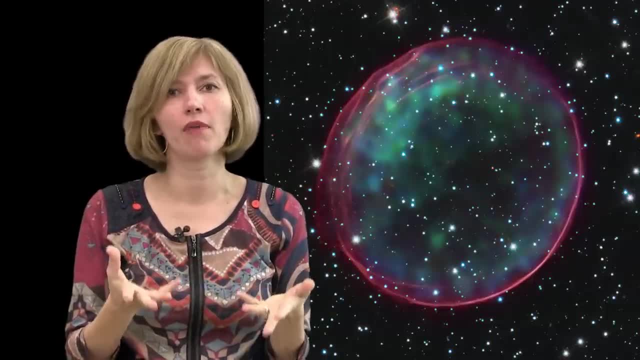 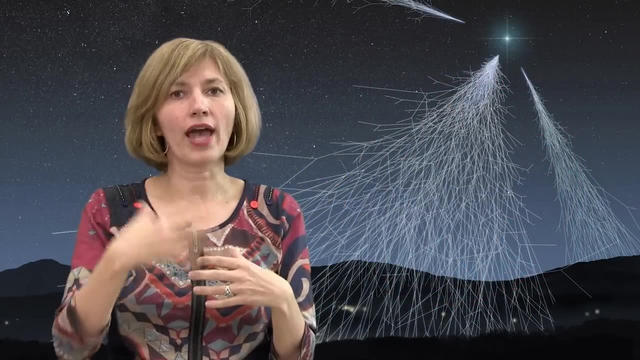 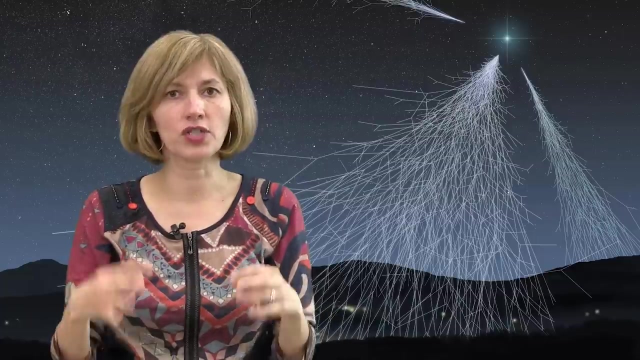 The only thing they're really responsible for is basically bombarding Mars with a lot of particles. So as the cosmic rays fall all over the sky, they interact with our atmosphere and they create a shower of particles. So by the time some of those particles reach the ground, they're quite low energy, So they're not as damaging. they're not ionizing radiation, So higher in atmosphere they are. this is why pilots and other people who fly are exposed to radiation a bit more, And this is why we have to limit how much time they spend high in.